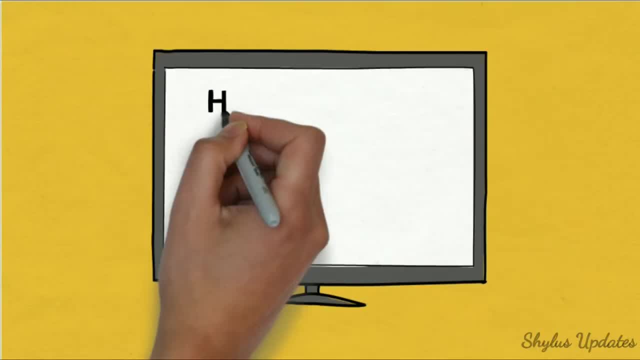 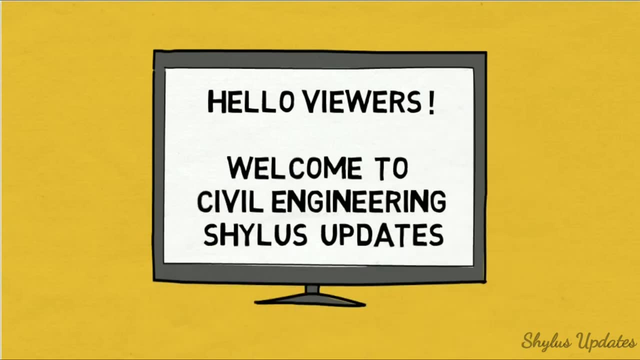 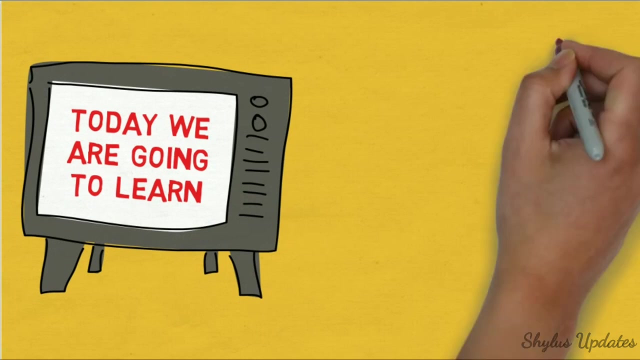 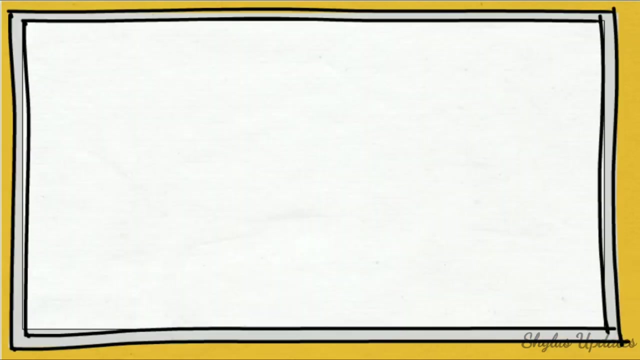 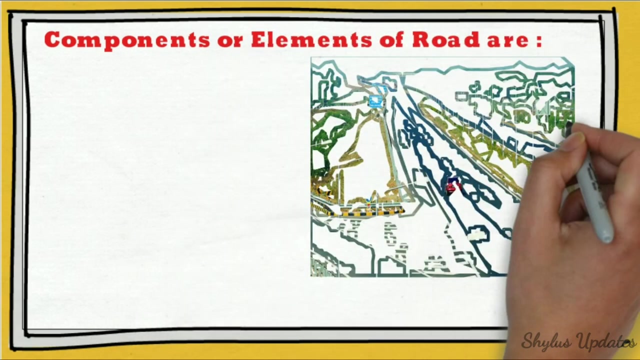 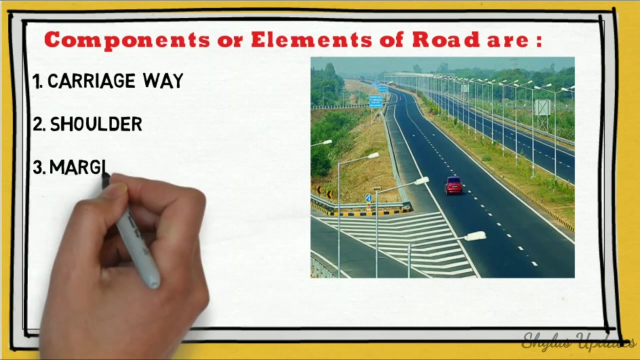 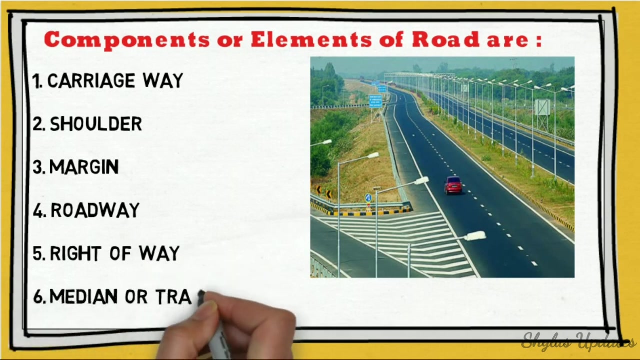 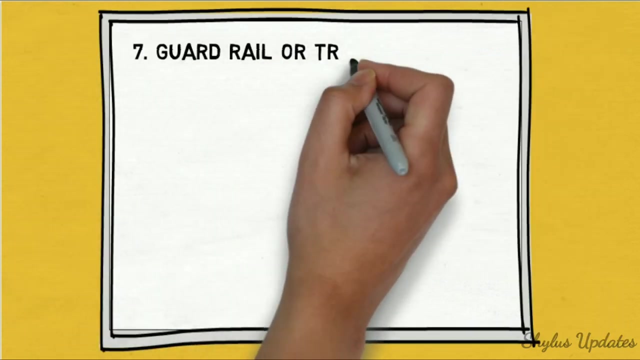 Hello viewers, welcome to civil engineering Shiloh's updates. Today we are going to learn road components. Components or elements of road are carriageway, shoulder margin, roadway, right of way, median or traffic separators, guardrail or traffic barriers, curbs, bicycle and. 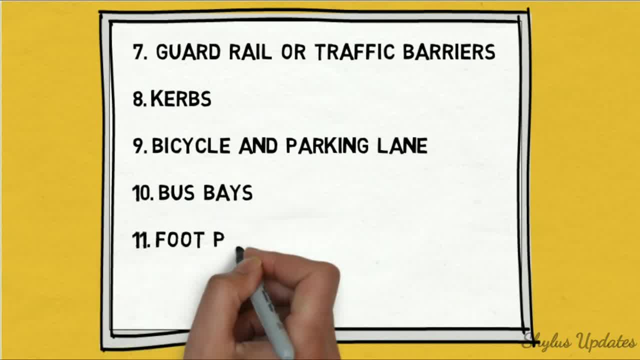 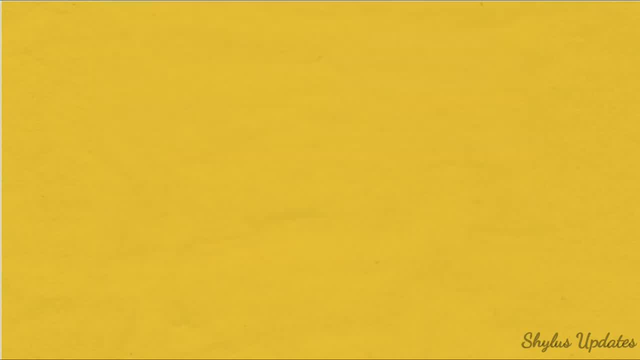 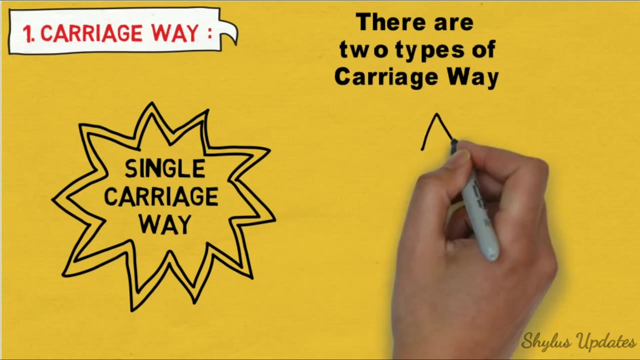 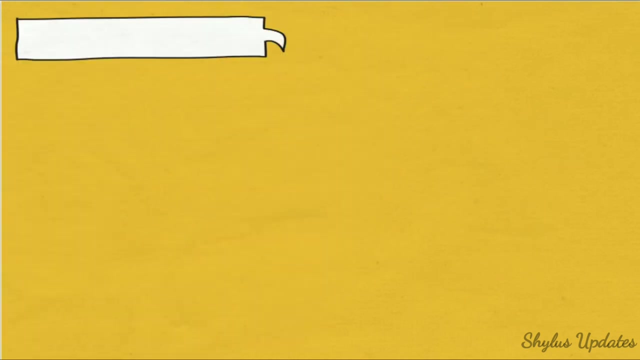 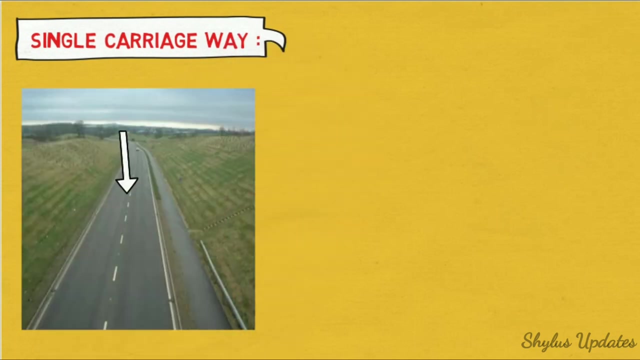 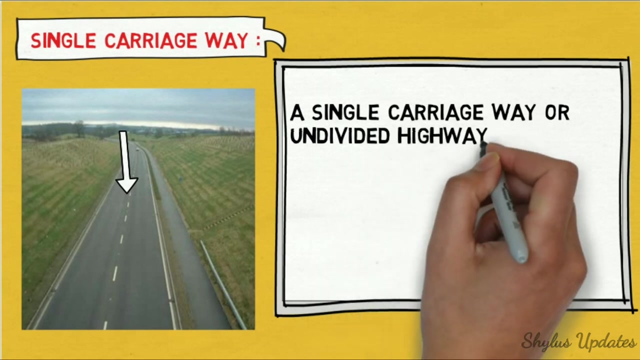 parking lane, bus base, footpath or sidewalk, camper Carriageway. There are two types of carriageway: single carriageway, dual carriageway. first let us see single carriageway. a single carriageway or undivided highway is a road with one, two. 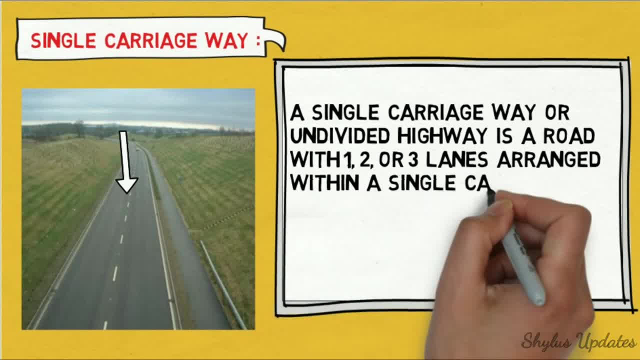 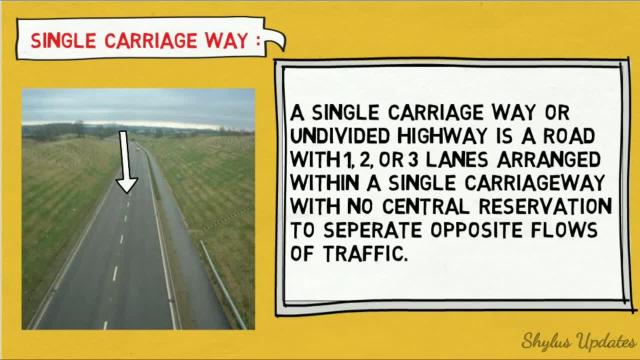 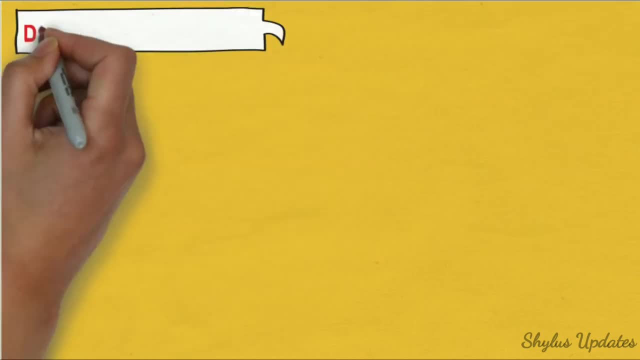 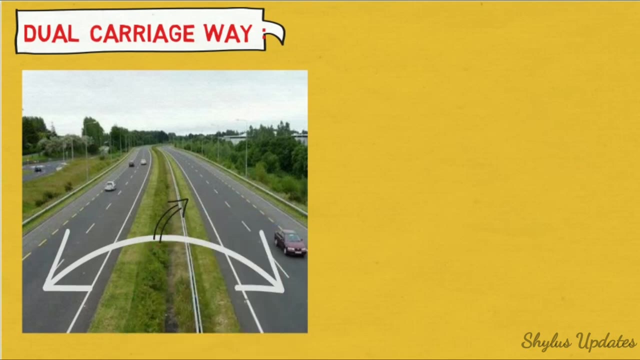 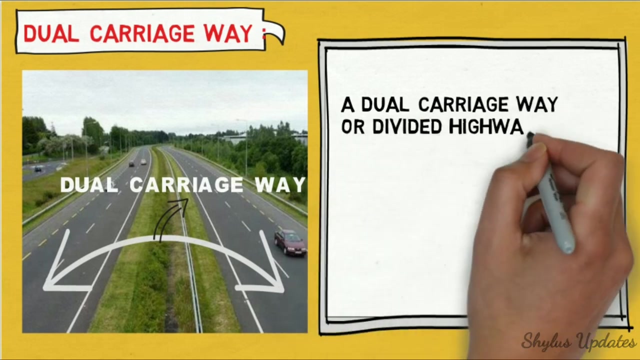 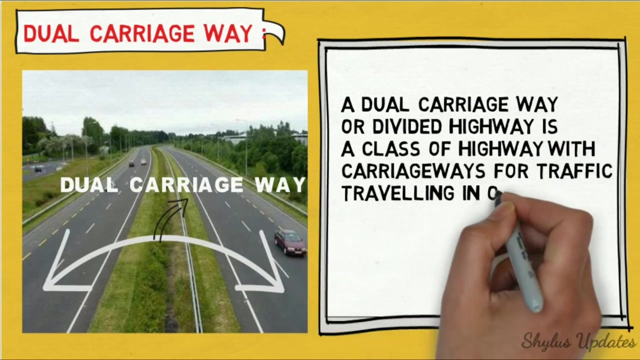 or three lanes arranged within a single carriageway with no central reservation to separate opposite flows of traffic. dual carriageway- a dual carriageway or divided highway is a class of highway with carriageways for traffic traveling in opposite directions separated by a 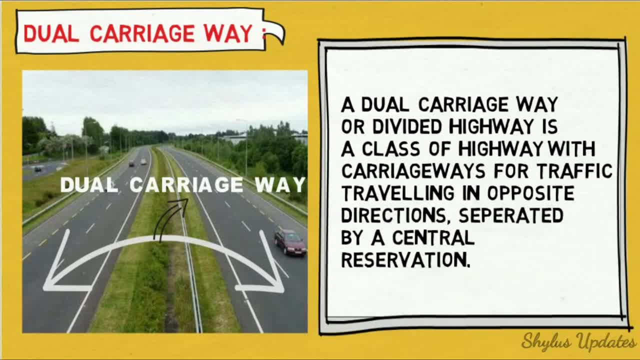 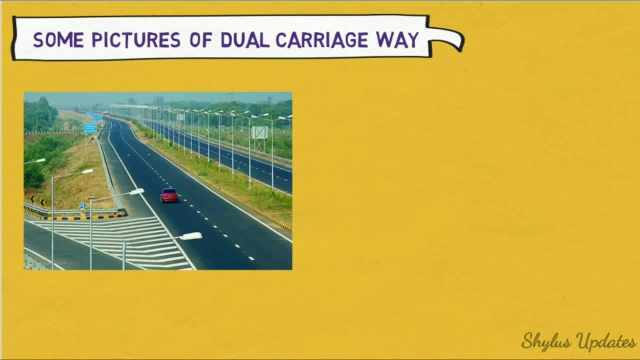 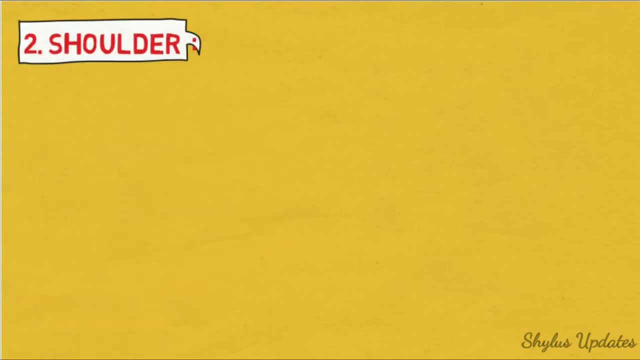 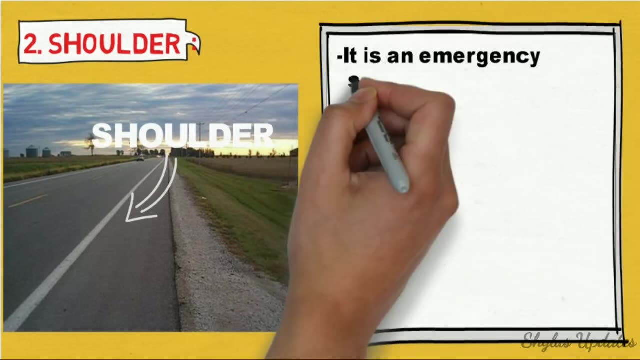 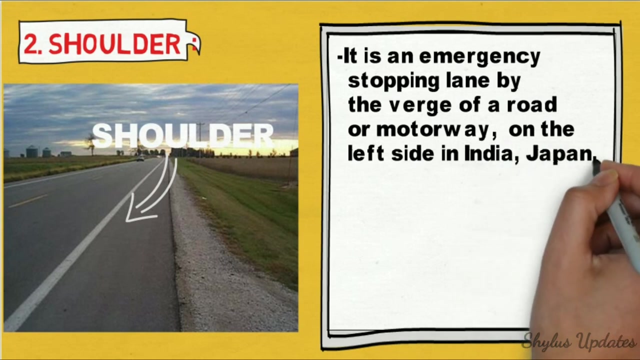 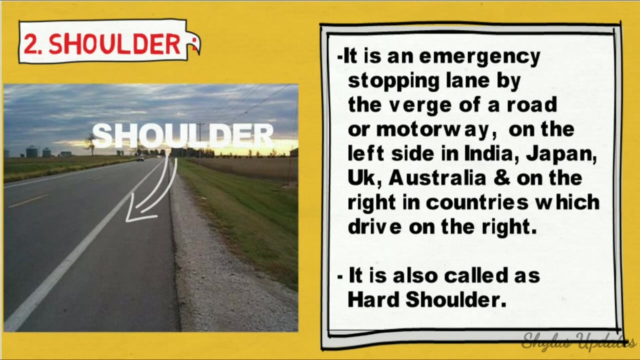 central reservation. Some pictures of dual carriageway soldier. it is an emergency stopping lane by the worse of a road or motorway on the left side in India, Japan, UK, Australia and on the right in which drive on the right. It is also called as Horde soldier. 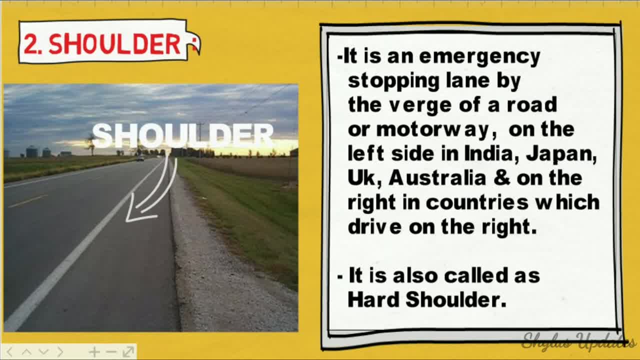 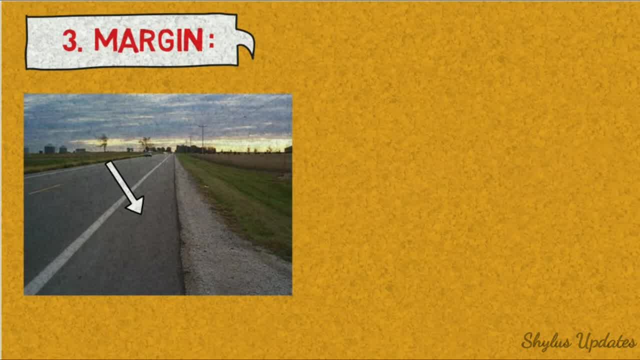 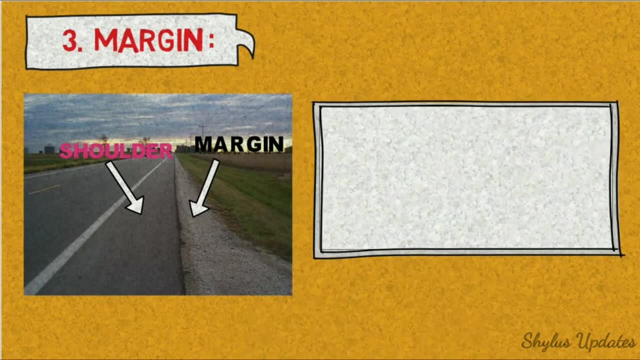 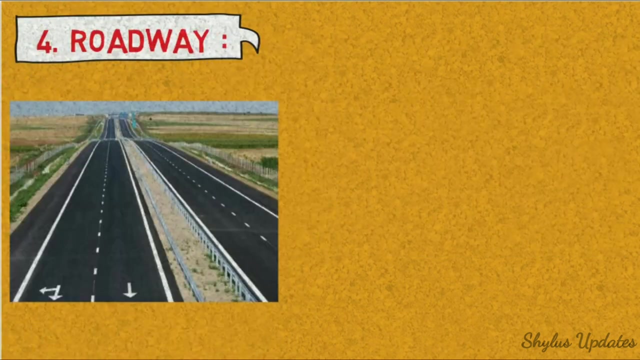 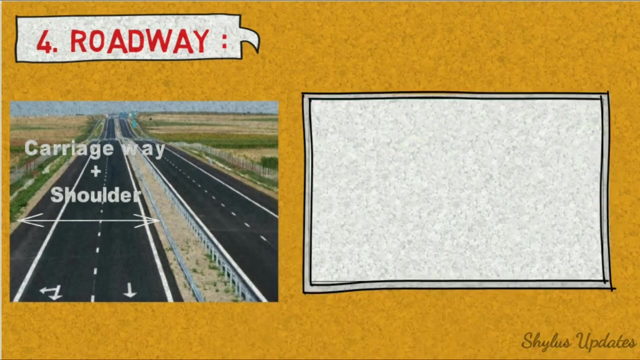 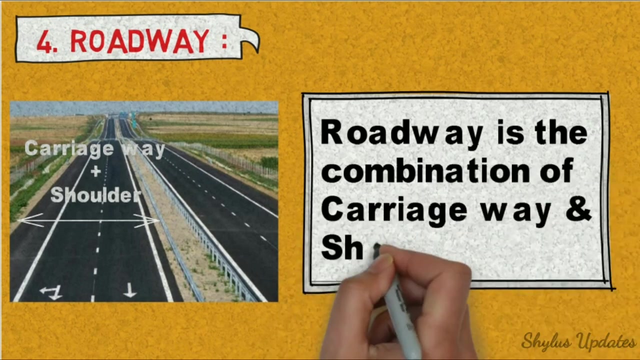 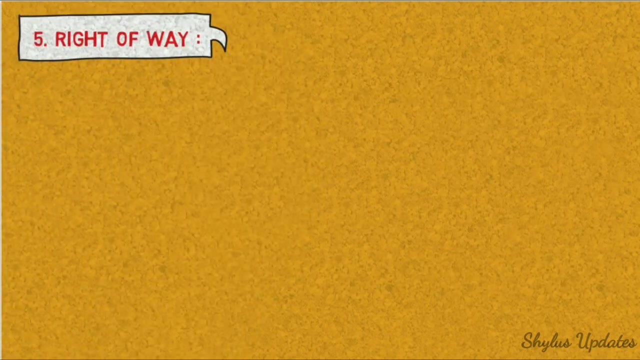 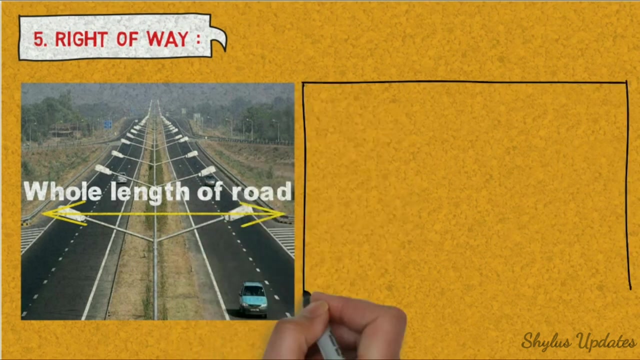 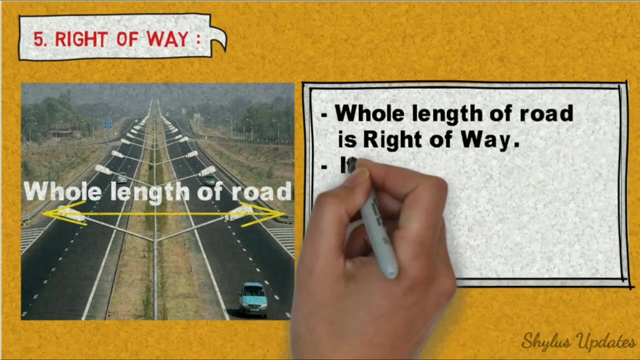 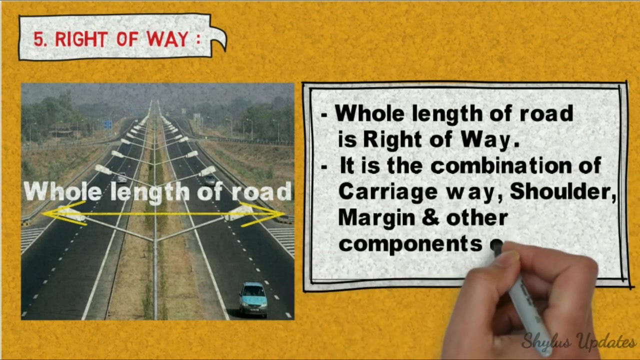 Margin. It is the small portion of the road provided after soldier Roadway Roadway. Roadway is the combination of carriageway and soldier Right of way. Whole length of road is right of way. It is the combination of carriageway, soldier, margin and other components of road. 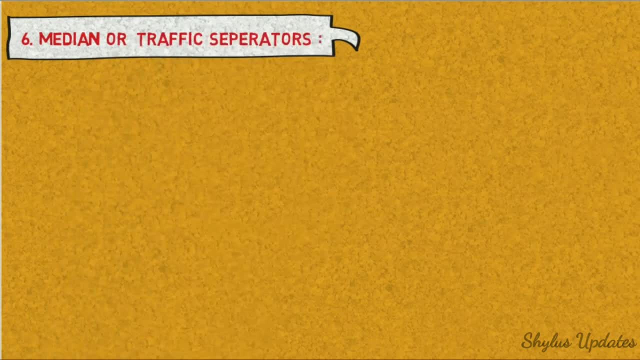 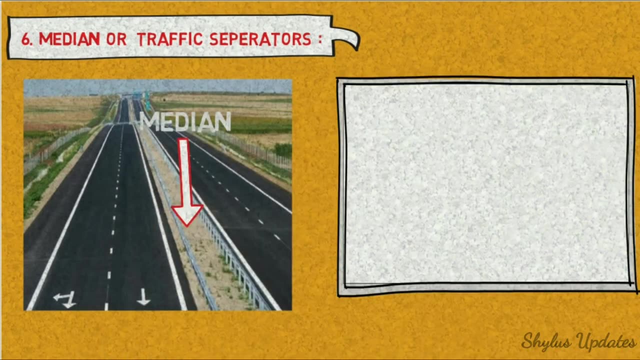 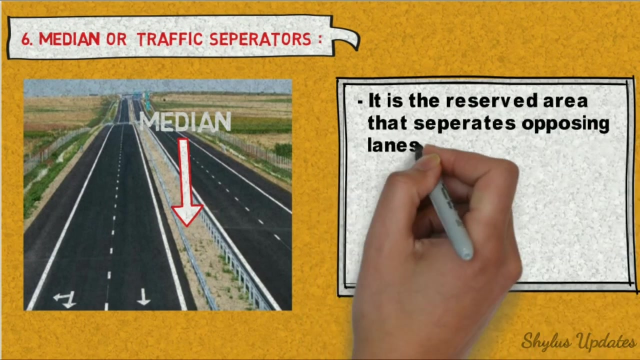 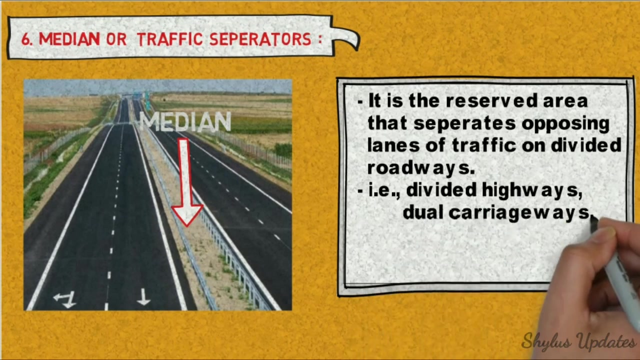 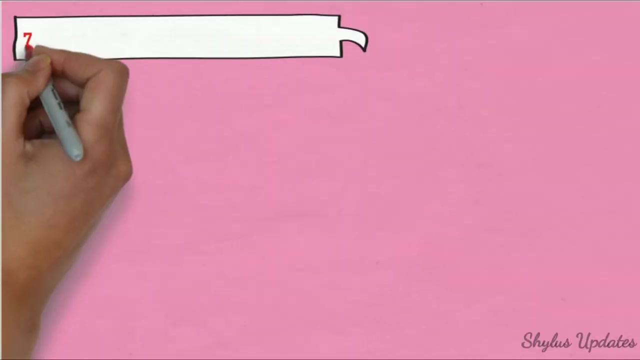 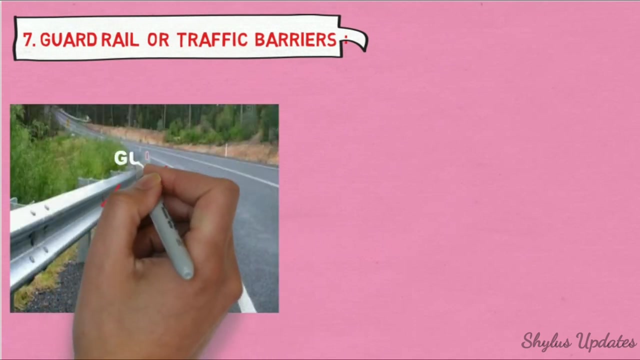 Median or traffic separators. It is the reserved area. It is the reserved area that separates opposing lanes of traffic on divided roadways, That is, divided highways, dual carriageways, freeways and motorways. Guardrail or traffic barriers. Guardrail or traffic barriers. 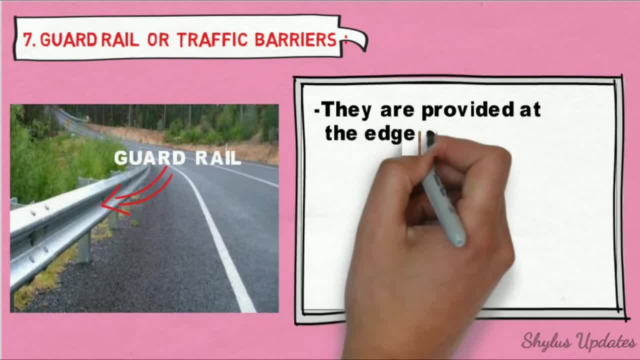 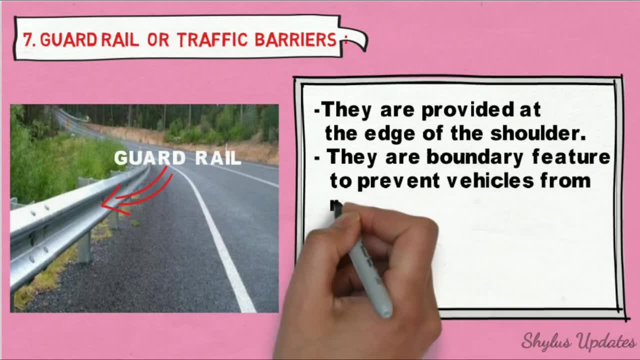 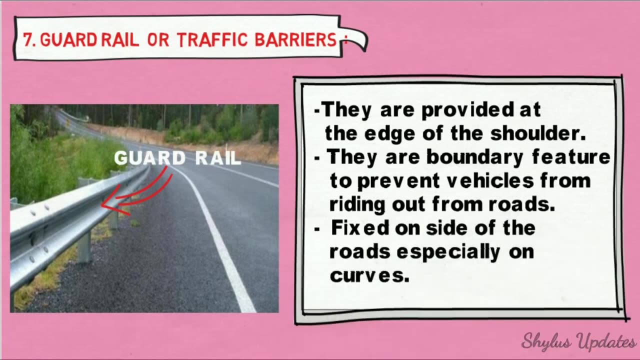 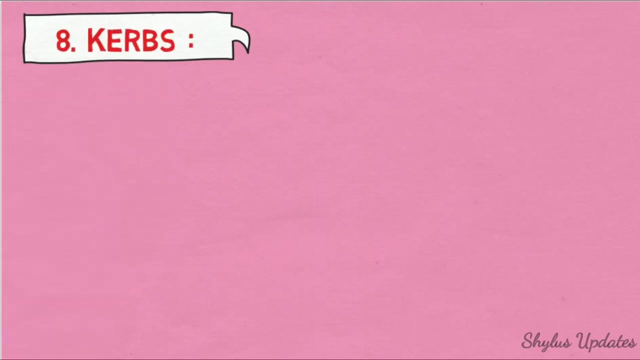 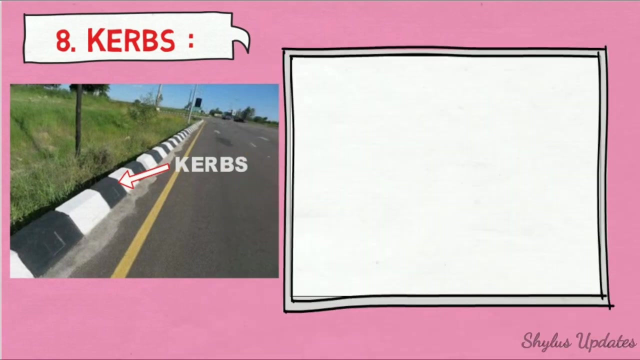 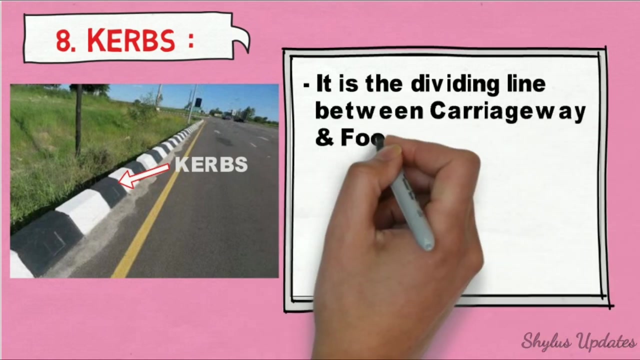 They are provided at the edge of the soldier. They are boundary feature to prevent vehicles from riding out from roads. It is fixed on side of the roads, especially on curves, Curves, Curves, Curves or barely. It is the dividing line between carriageway and footpath. 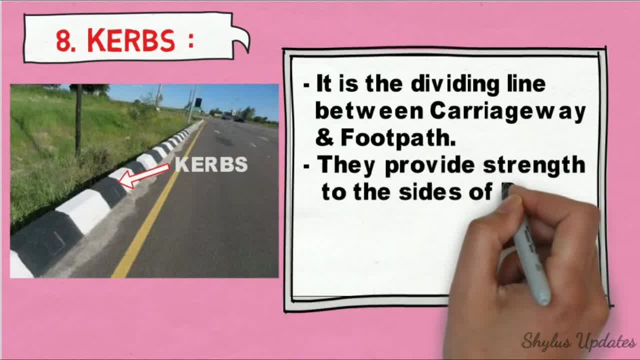 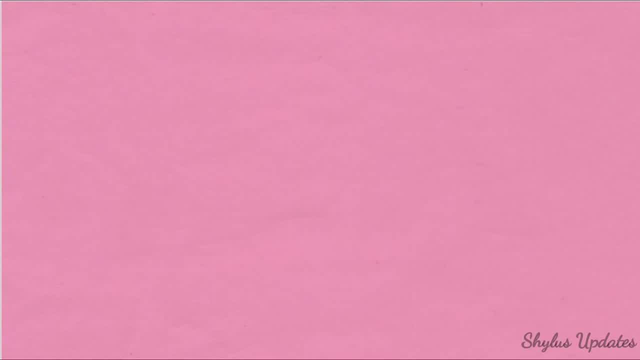 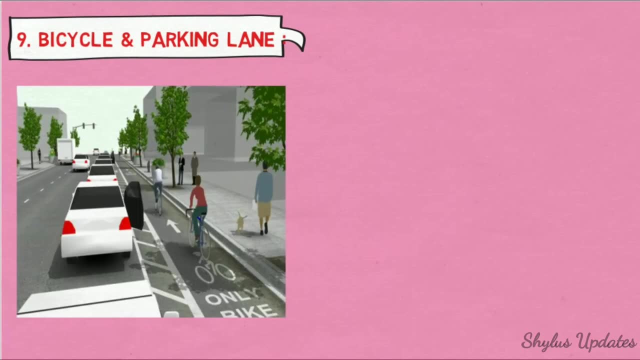 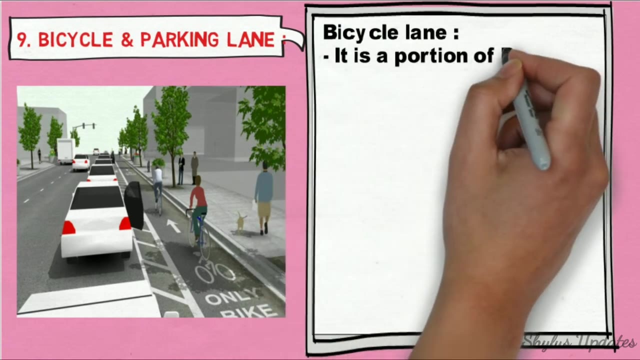 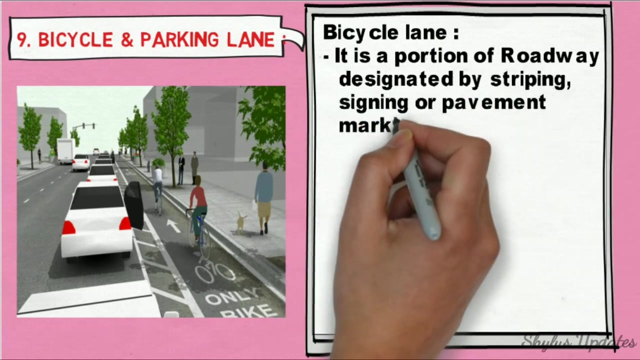 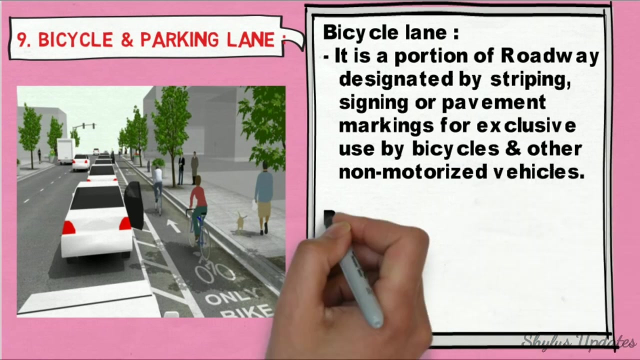 They provide strengths to the sides of road pavements. They aid Bicycle Lane: It is a portion of roadway designated by striping, signing or pavement markings for exclusive use by bicycles and other non-motorized vehicles. Parking Lane: It is an additional lane provided on urban. 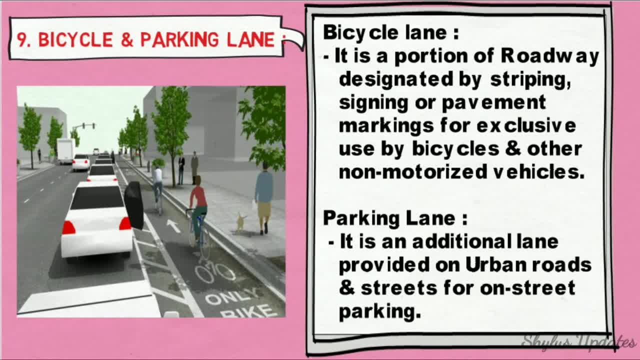 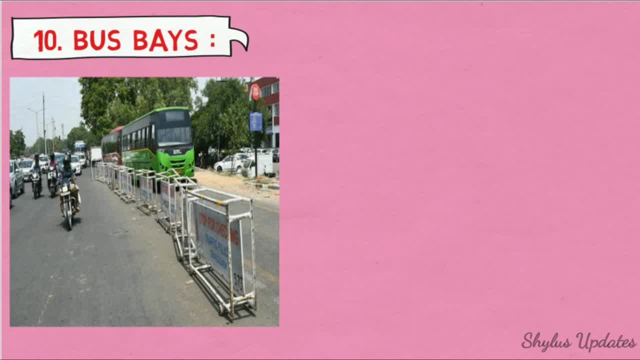 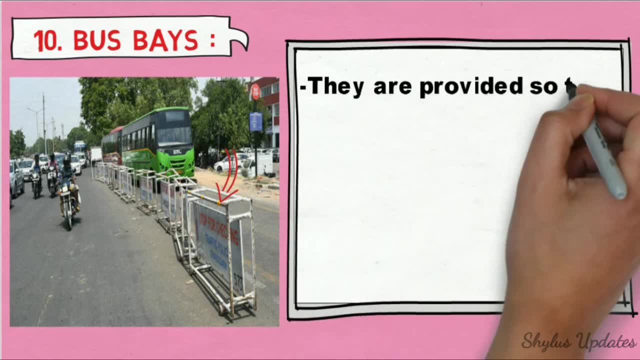 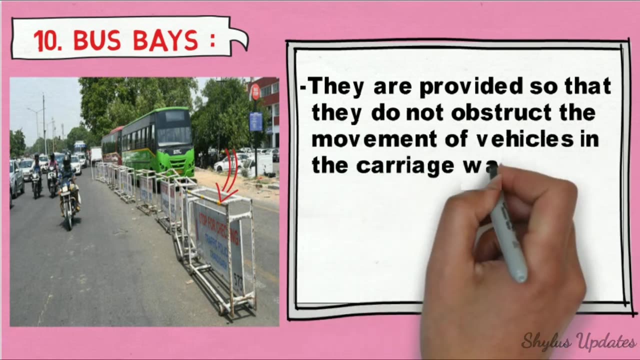 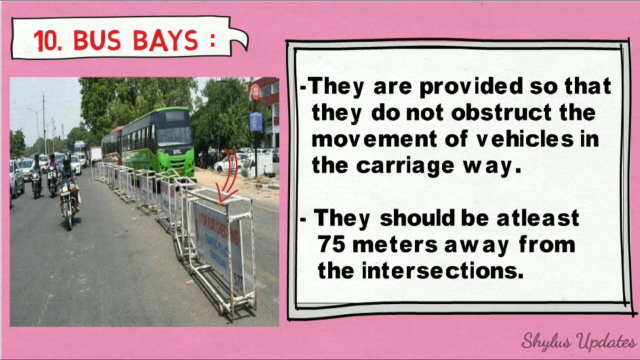 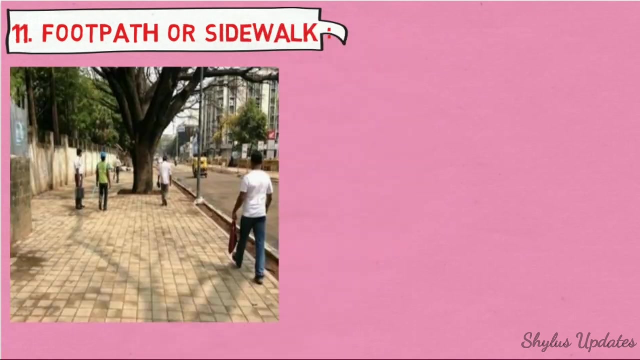 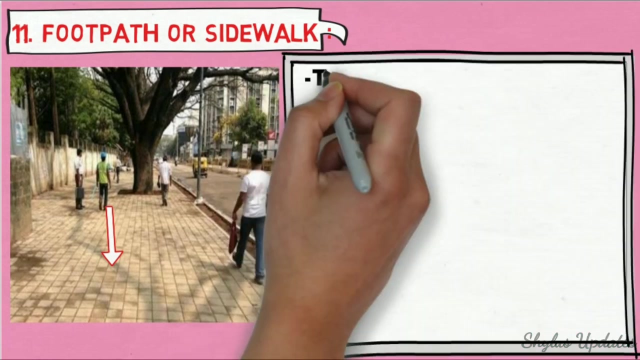 roads and streets for on-street parking Bus Bays. They are provided so that they do not obstruct the movement of vehicles in carriageway. They should be at least 75 meters away from the intersection Footpaths- Footpaths are sidewalks. 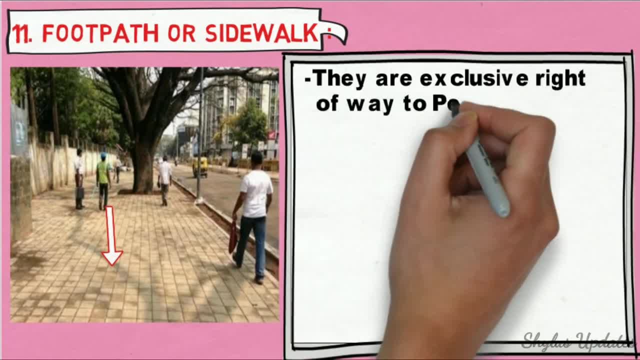 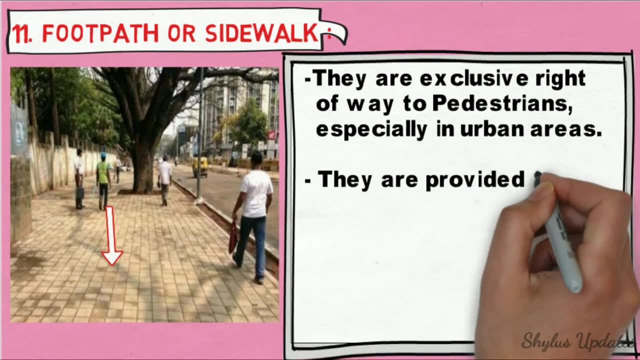 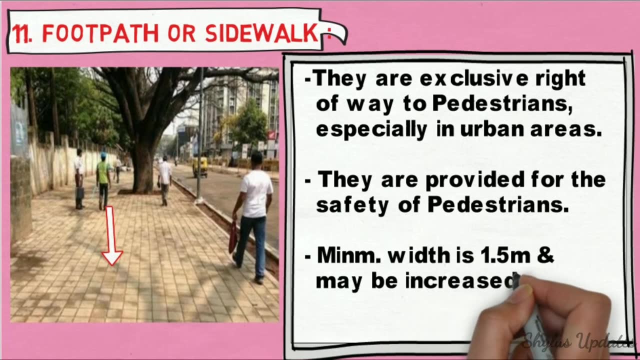 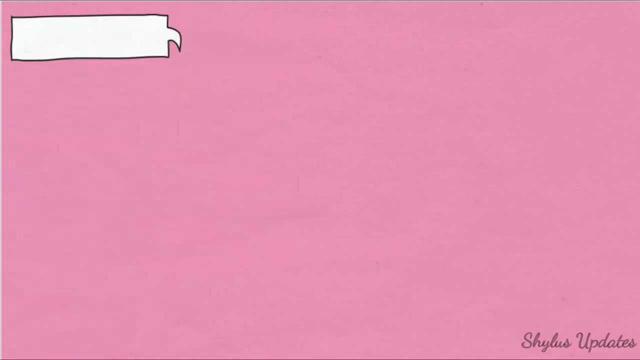 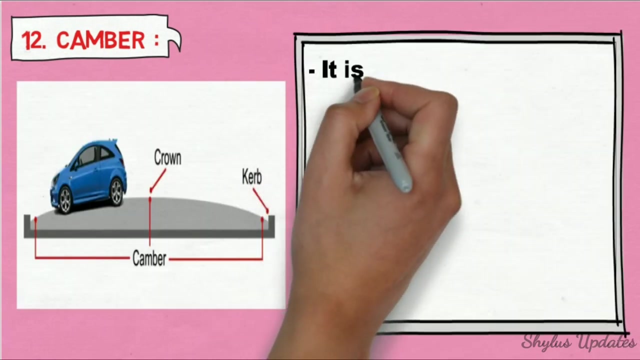 They are exclusive right-of-way to pedestrians, especially in urban areas. They are provided for the safety of pedestrians. Minimum width is 1.5 meters and may be increased based on the traffic Camper. It is the slow provided to the road surface. 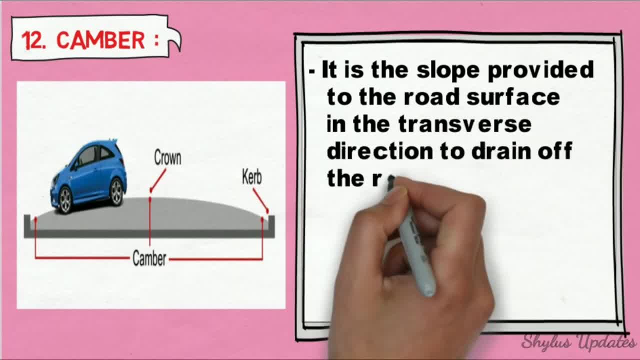 in the transverse direction. They should be at least 75 meters away from the intersection. They are provided so that they do not obstruct the movement of vehicles. in carriageway, Minimum width is 1.5 meters and may be increased based on the traffic.